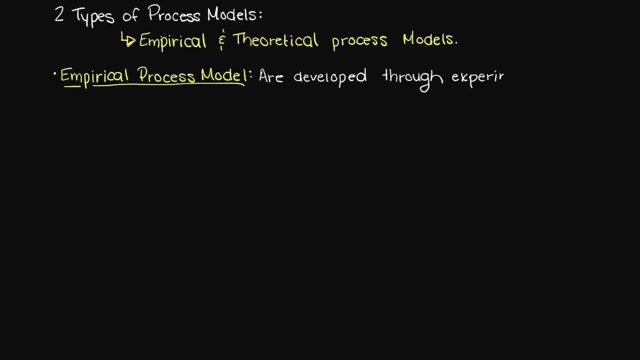 Let's begin with what an empirical process model is. Empirical process models are developed through experimenting on the actual system or something physically close to the actual system, So our data for our process model is coming from an actual experiment we would perform. Let's think of an example to better understand this, though. 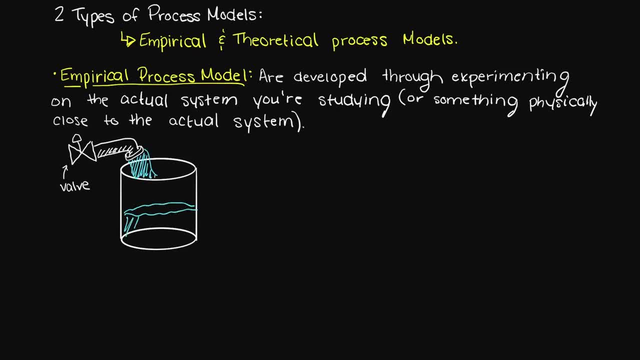 Let's say that we are looking to develop a process model for a bucket that is filling with water at various inlet flow rates. We could do the following: Open the tab 10% and see how long it takes for the water to fill our bucket and then say: repeat this for 20%, 40% and 60%. 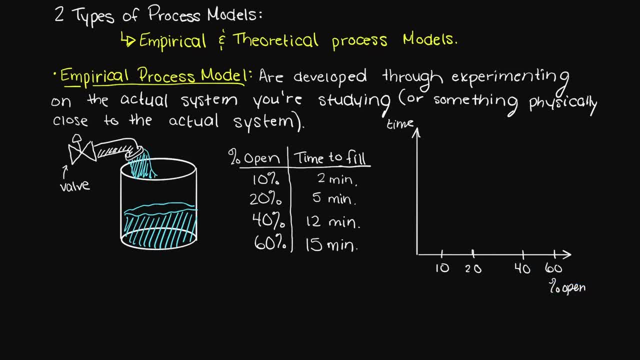 This would give us an idea of how the system performs under those conditions. This allows us to see how the system performs under those conditions. This allows us to keep our math as simple as possible and gives us more control over our experiment and the ranges that we wish to perform our experiment over. 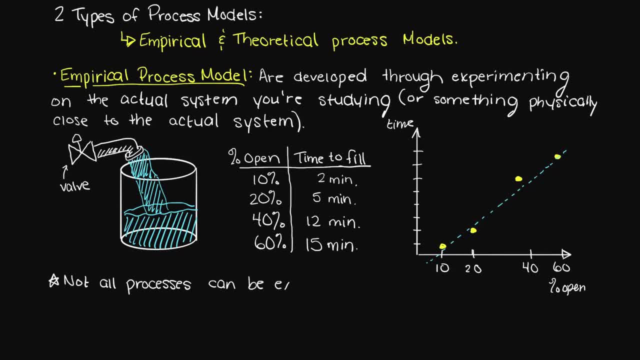 The drawback to this process development method is that not all processes can be experimented on Typically. this is either because they are too expensive or too risky, And we can only really reliably use our exact experiment data to work off of, as the data likely won't extrapolate very well. 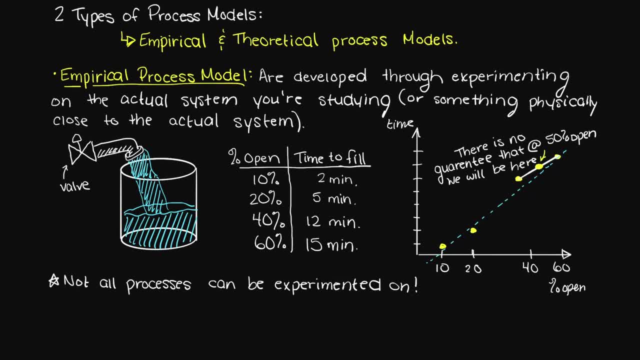 By that I mean that even though we tested our tab at 40% and 60% opened, there's no guarantee that at 50% we will be right in the middle of those two values, And if we fail to account for this in our final control system, this could be a very costly mistake. 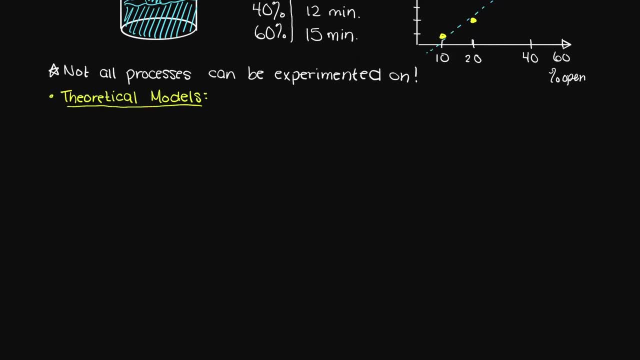 Now let's talk about theoretical models. Well, unlike empirical models, these strictly rely on first principles and the physical laws such as conservation of mass energy and momentum. Because of this, the math will become more complicated than empirical models. 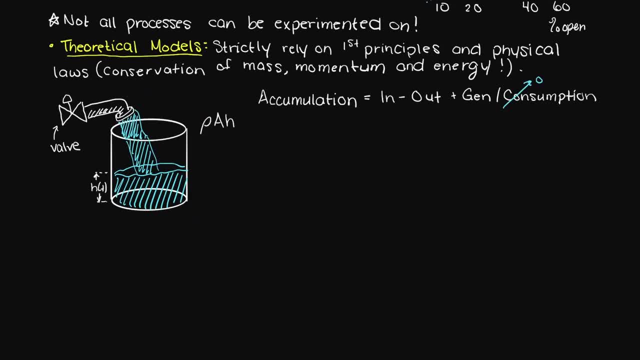 However, because the math is derived straight from laws and principles that we know and trust, we can reliably use our data over any given input. So in our previous example, if we developed some theoretical model for the tab filling our bucket, we could trust our model from 0% to 100%. tab opening. 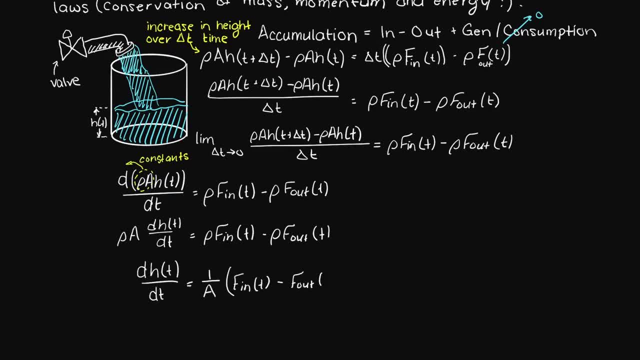 This type of process modeling is also excellent for trying different designs and operating conditions, whereas an empirical model would require much more work and experimentation. However, the theoretical models are not without their own drawbacks, Like I previously stated, the major drawback to this method of process modeling: